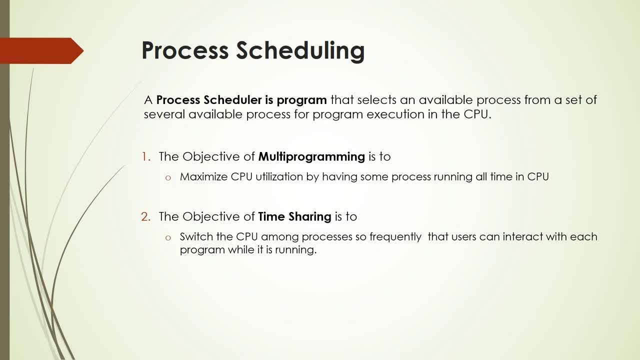 process so frequently that the user can interact with each other while it's running. So that is why we need process scheduling. So the scheduler program is responsible for scheduling the processes, That is, which process will execute first, which will execute second, and so on. 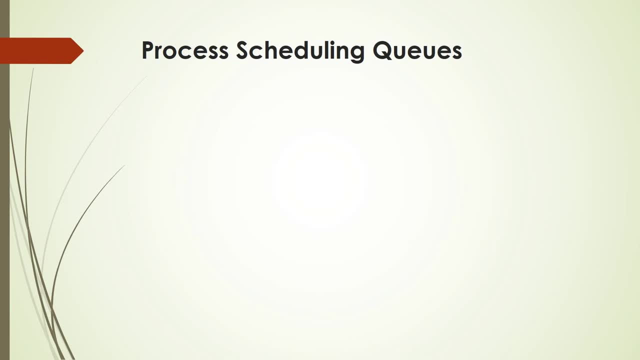 Now let us look at process scheduling queues. As there are several processes, so all the processes are put in queue so that they can be executed in some order. So the first queue is called job queue. Then all set of processes in the system are put in the job queue. Second, ready queue. 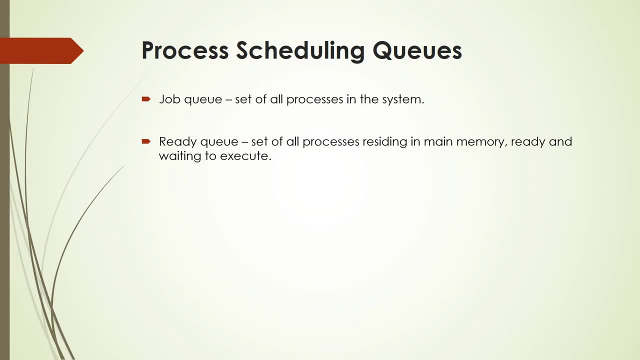 The set of all processes residing in main memory and that are ready and waiting to be executed. Third device queue: The set of processes waiting for input output operation or input output devices, And the processes migrate between one queue to another queue. For example, it: 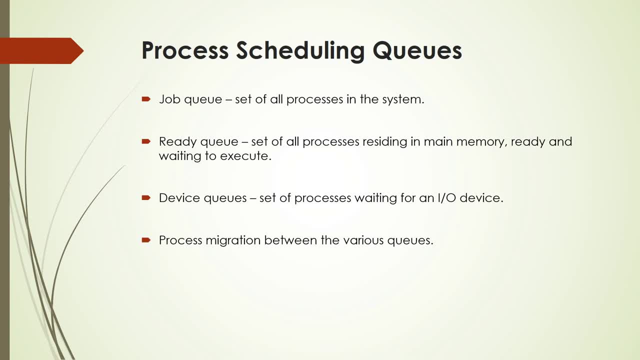 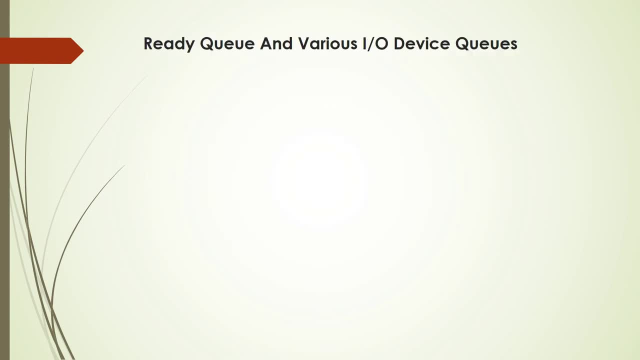 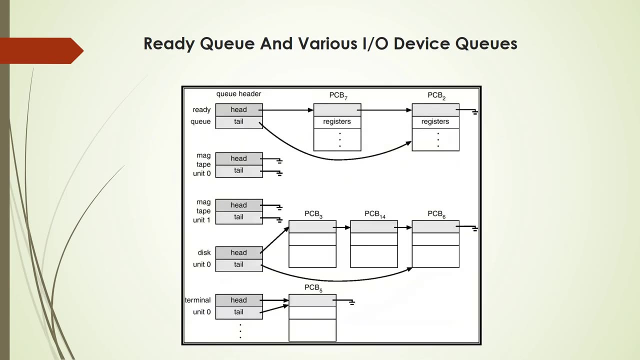 may move from job queue to job queue, queue to roadie queue, then to device queue, or from ready queue to device queue, device queue to back to ready queue, and so on. so let us look at the example of ready queue and various input output device queues. so in the example, if you see the first one, we 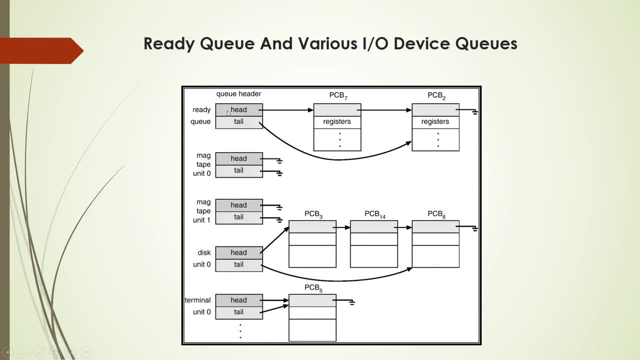 see, this is a ready queue and there are two processes in the queue: process seven and then process two. so they are represented using their pcb process control block. so process control block for process seven and process control block for process two. and if you see the queue, the first process in the queue is represented by this particular pointer head. 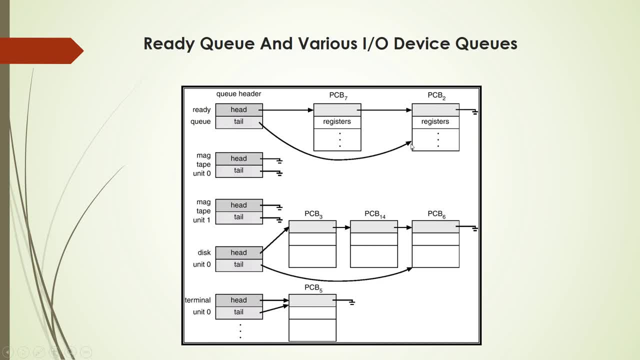 and the last process is represented by the pointer tail. so in between there can be several processes. so each process will contain again a pointer to the next process in the list. similarly you can see there is a device queue for magnetic tape and the head and tail. if you see, initially these are null. there is also disk unit which 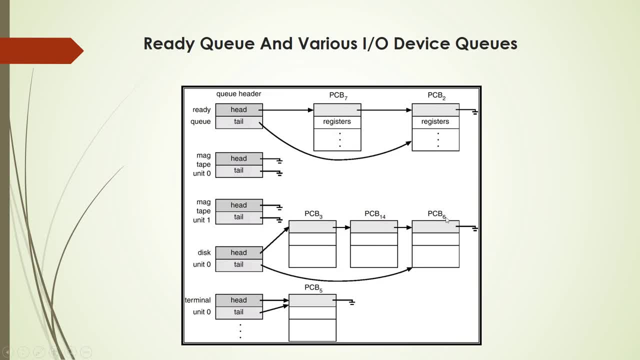 has three processes: process three, process fourteen and process six, and the head is pointing to the first process and the tail is pointing to the last process. in between, there can be several processes, as shown here: that process three, after that process fourteen, then after that process six, and they are all represented using process. 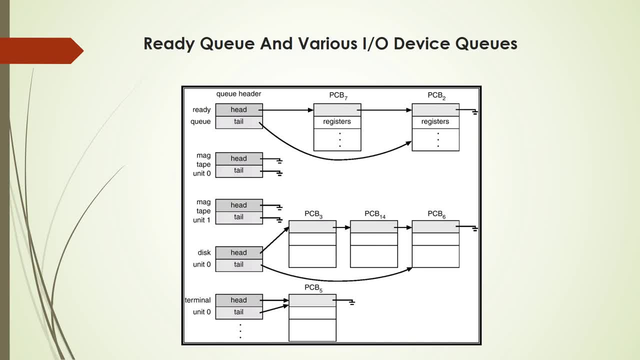 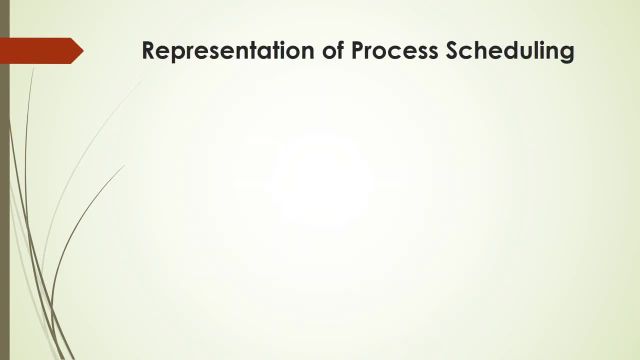 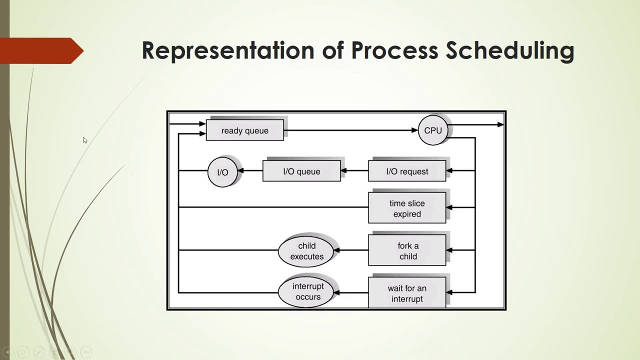 control block. so pcb contains all the information associated with a process, representation of process scheduling. so let us look at this particular example and understand how process scheduling takes place. so initially there is a job queue, all the processes are in their job queue, and then they are moved to the ready queue. 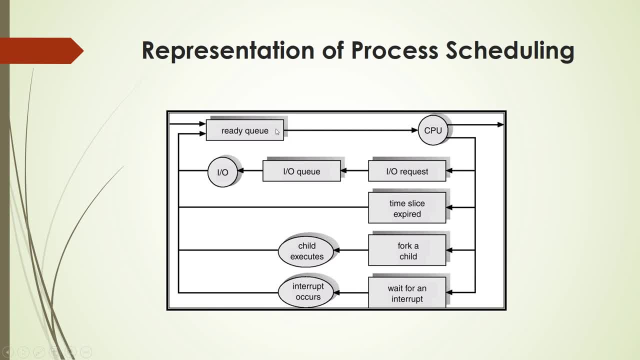 now you know already that queue works in first in first out manner. the process which comes first will be executed first, the process which comes last will be executed last. so all these processes are now in the ready queue. now the first process will be moved to the cpu for 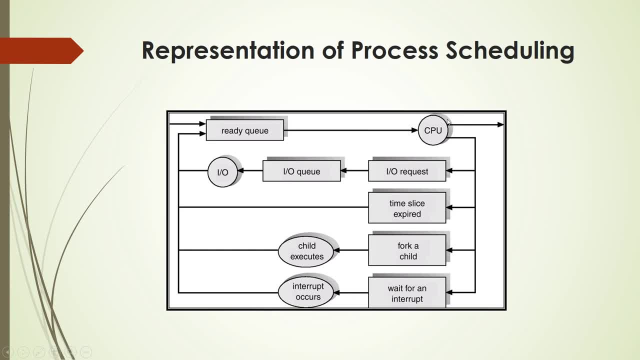 execution. now, while the process is in execution in the cpu, there can be several possibilities. one of the possibility is that there is a input output output instruction in the program or in the process, so the process will need a input output so it cannot run in the cpu. so that is why it will be halted and it will go for a input. 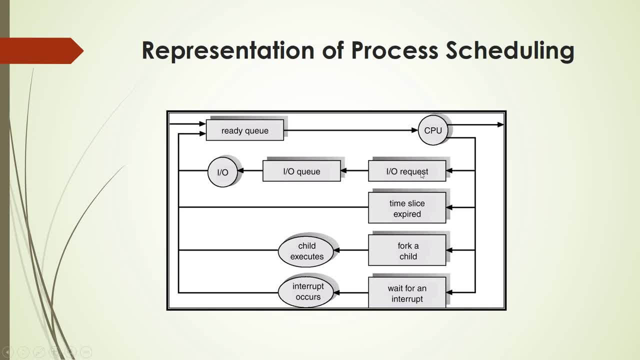 output request. now because input output request. there can be several devices which can need input output so it has to go to a input output device queue. so after the input output request has been granted to that particular process it will execute in the input output, for example taking a input from the user, and then it goes back to the ready queue or there is a possibility. 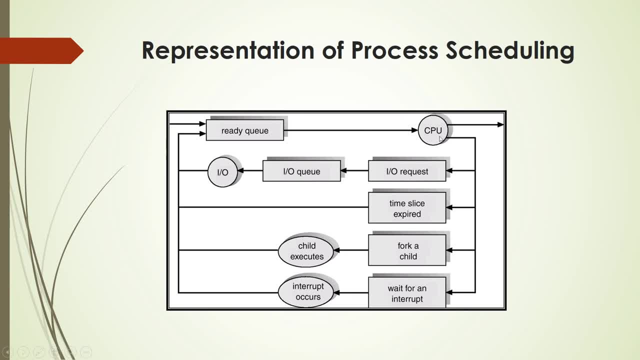 that the cpu in which the process is running there is a time slice, that is, the process will run for a certain duration of time. after that time it will be taken out of the cpu and the new process will get a chance, or the second process will get a chance. generally, every cpu maintains a time slice. why this time? 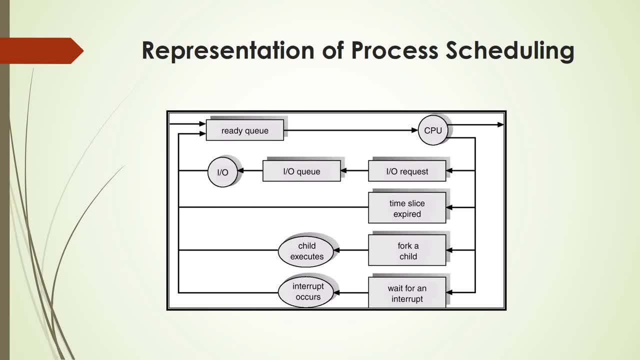 slice so that every process gets the equal opportunity. so for example: first, two millisecond can be given to process one, second, two millisecond can be given to process two, third, second, second, two milliseconds can be given to process three, and so on. so there can be several processes. 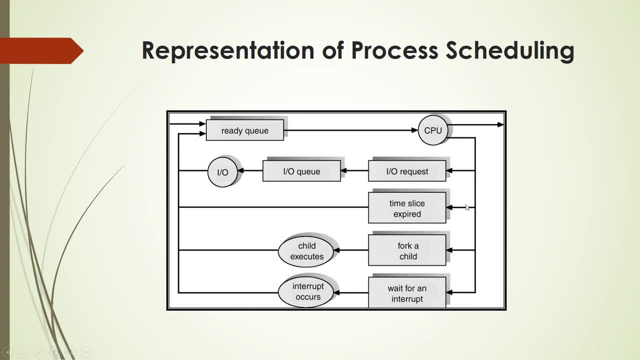 each given two milliseconds so they may go to the ready queue, to the cpu. then they can be taken out from the cpu because their time expired and then they goes back to the ready queue again. so the process may run several times through the ready queue and finally, 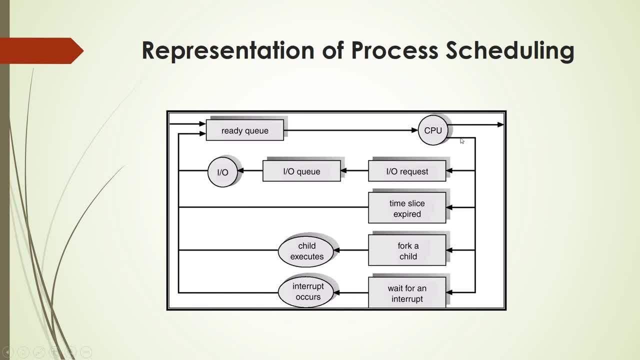 it may complete its execution. so it will come out. also there is a possibility that the process may create a new process. so when a process creates a new process, in that case it is again taken out of the cpu. so when the child process because process- is created a new process, which 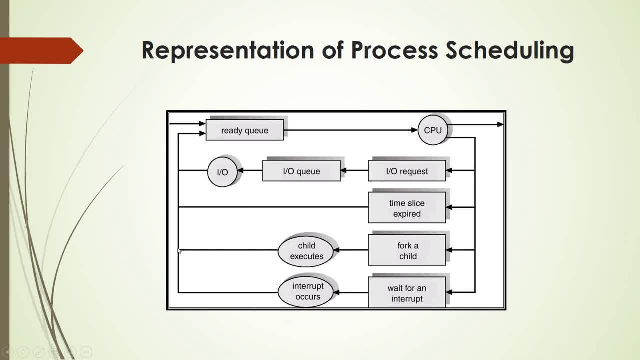 is also called the child process. so when the child process completes its execution, then the parent process can continue its operation. so in that case, because a new process is created, it will go to the ready queue and will wait for its turn. also there is a possibility of interrupt. so when the 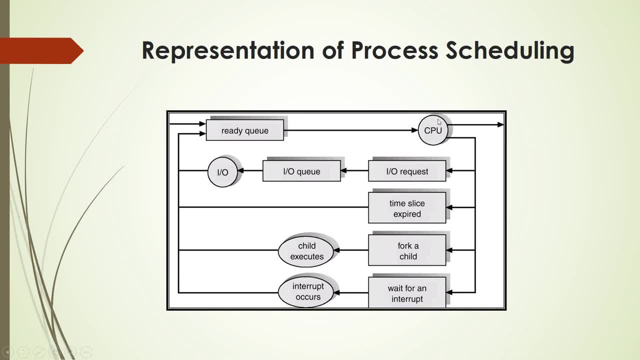 process is executing in the cpu, there may be an interrupt from the operating system. so in that case the last option, wait for interrupt. so the process will be taken from the cpu and it will wait for the interrupt to finish when the interrupt routine or interrupt program has finished its execution. 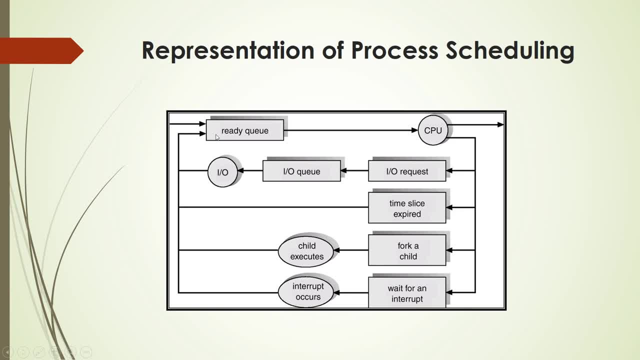 then it will go back to the ready queue and again wait for its chance. so if you see, there are four possibilities in which a running process in the cpu will be halted. one is the input output request. second, the time slice: the duration of time for which it will run. 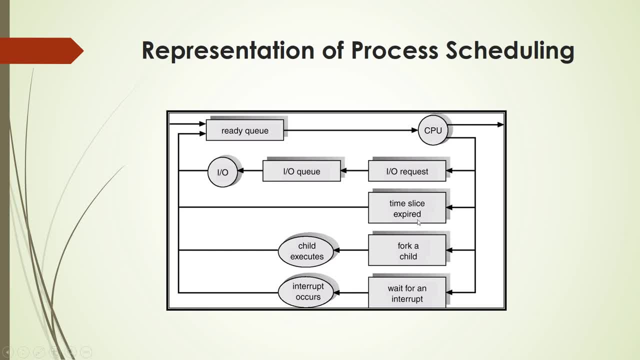 in the cpu. once it has expired it will taken out. the third: the process has created a new child process, so the child process must run. and fourth, there is an interrupt from the operating system so the process has to wait for the interrupt to finish. so these are the four possibilities when a process is running in the cpu, so that 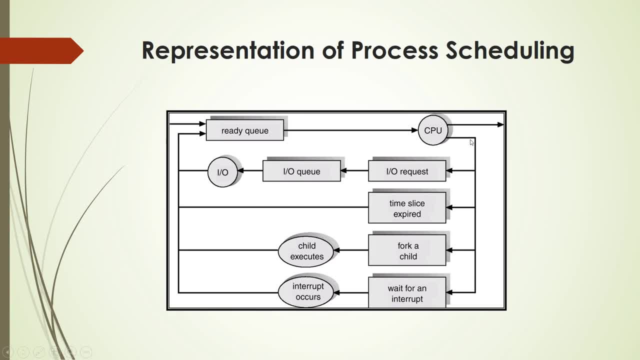 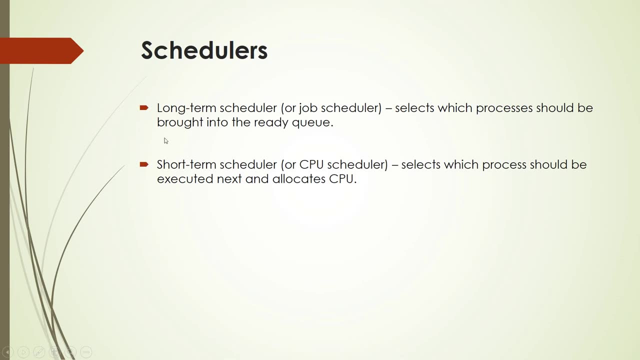 is why we need a scheduling, so that in each of these cases it goes to the ready queue and then it moves back to the cpu. next we see scheduler. so generally there are two types of scheduler. one is called long term scheduler and another one is called the short term scheduler. long term scheduler is also called 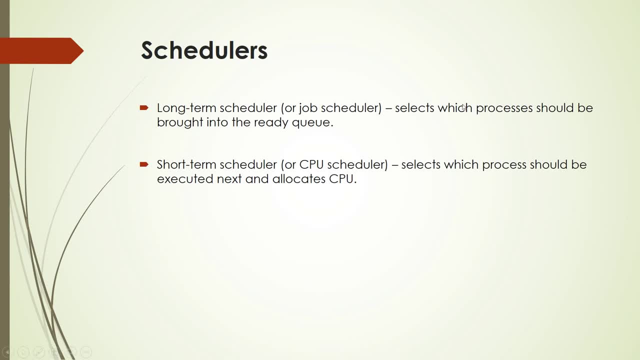 job scheduler. so the long term scheduler selects process which should be brought into the ready queue, so from the job queue it is brought to the ready queue. and the short term scheduler, which is also called the cpu scheduler, selects which process should be executed next and allocates. 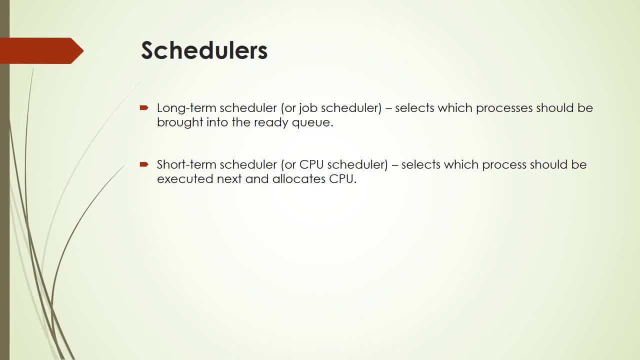 the cpu. so the long term scheduler will bring the processes from the job queue to the ready queue and the short term scheduler will move it from the ready queue to the cpu and then back to the ready queue, then cpu, and the process will continue until the system or the scheduling 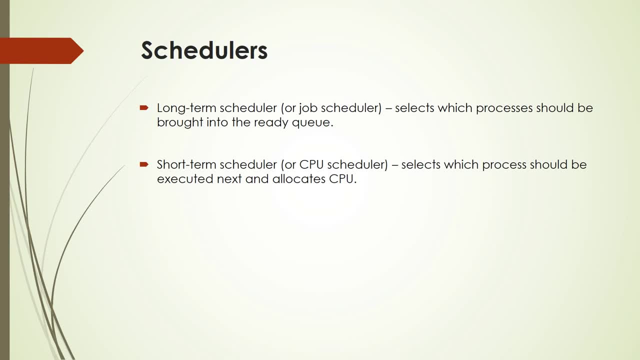 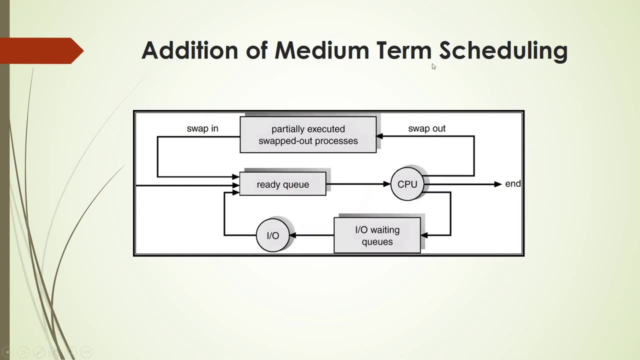 program finishes the execution of the particular process. there is also one more scheduler, or the scheduling program or scheduling technique, which is also termed as medium term scheduling. in this, if you see, the process is in the ready queue, it goes to the cpu and then after some time it is swapped out. 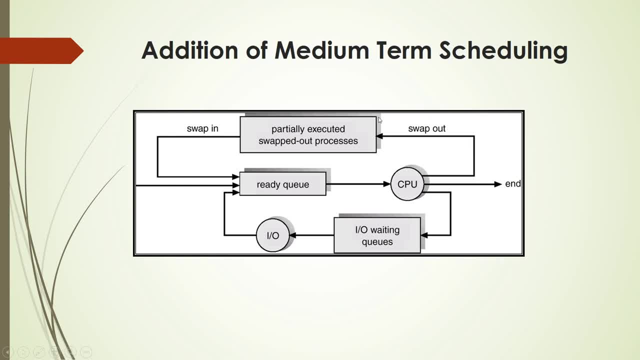 the process may have completed partially, so it will be swapped out and then it will be swapped in back to the queue. the main idea of this scheduler is that the process will continue until the system or the scheduling program finishes. the main idea of medium term scheduler is that 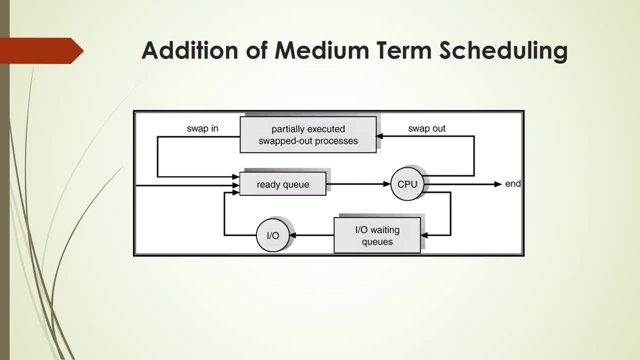 it is sometimes advantageous to remove processes from memory and reduce the degree of multi-programming. also, the process can be reintroduced into the memory at a later stage and can be made to continue from where it let off. this scheme is called swapping. the process of swapping in and out several times by the medium term scheduler is necessary to 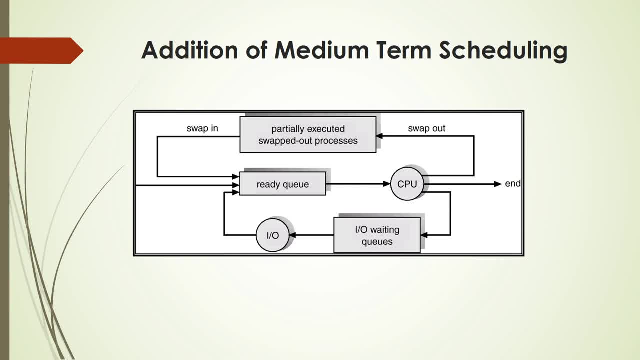 improve the process mix so that there are several processes and everyone get its chance also to change the memory requirement, as there may be a possibility that the memory needs to be made free, so the process needs to be taken out of the CPU. so that is why swapping is done in and out several. 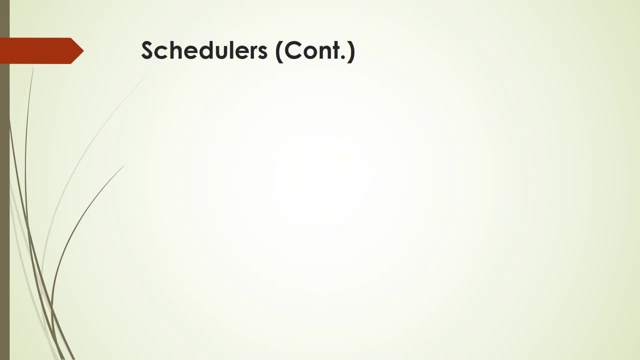 times. continuing with schedulers, short-term scheduler is invoked very frequently in millisecond and must be very fast. as you know, the process goes to the CPU, then to the ready queue and this switching takes place in a very short period of time. so the process needs to be taken out of the 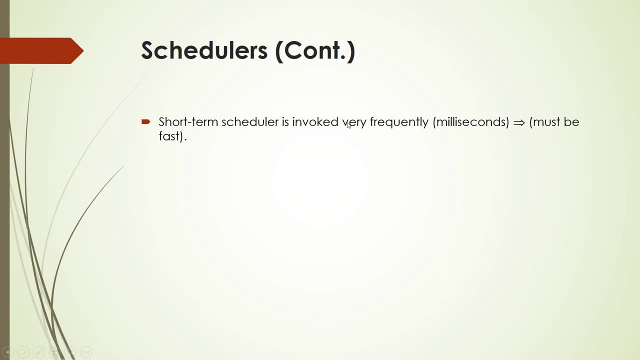 CPU. so that is why swapping is done in and out several times, continuing with schedulers short-term very frequently. that is why it has to be very fast. in case of long term scheduler, new processes will come in from the job queue to the ready queue, so the process may be little slow. the 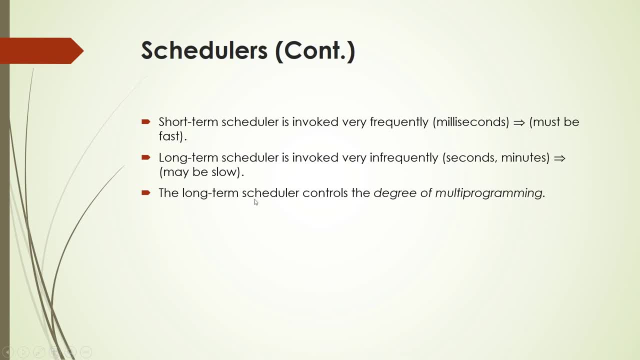 long term scheduler controls the degree of multi programming. multi programming concept we have already discussed, and there are two concept of multi programming: that the processes can be input-output bound processes or it can be CPU bound process. if it is input-output bound, that means it is spending more time in input-output operation. 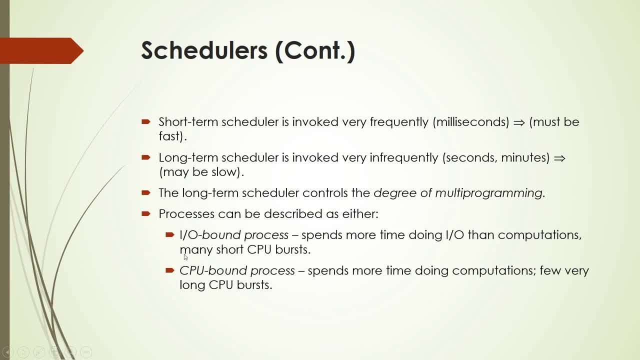 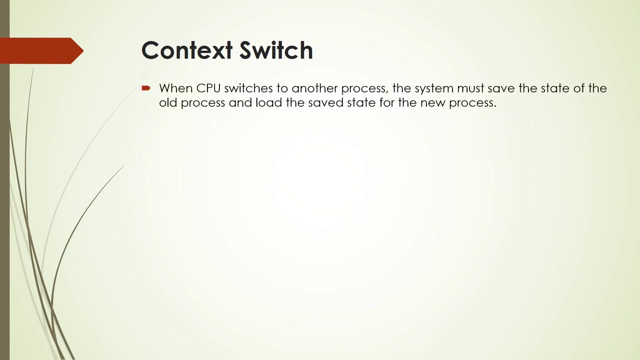 then it may need short CPU burst, that is, it will take less CPU time. some processes which are CPU bound spend more time in CPU whereas they will taking less time in the input output. so they will need long CPU burst or long CPU time. so that was about scheduler. coming to context, switch when CPU switches to one process to another. 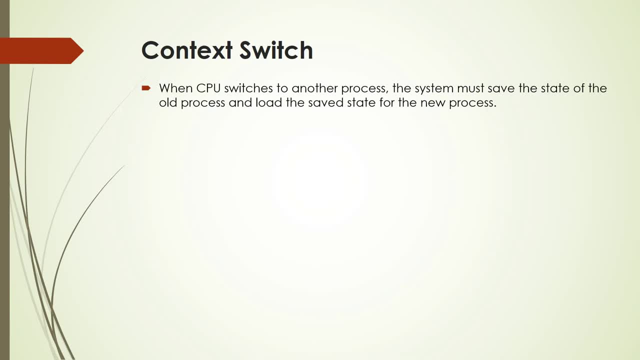 the system must save the state of the old process and load the safe state of the new process. we have already seen this in the last video lecture. when context switching time is overhead, the system does no useful work while switching. so when the CPU switches to the new process, the system must save.